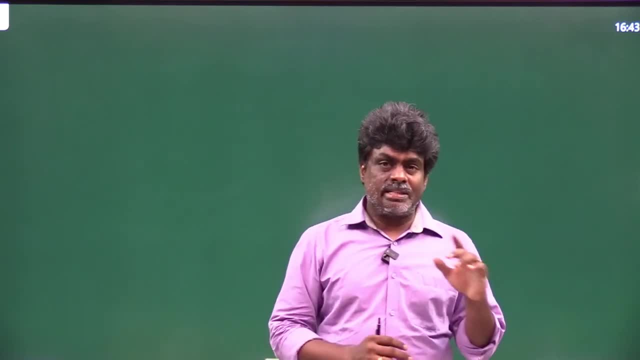 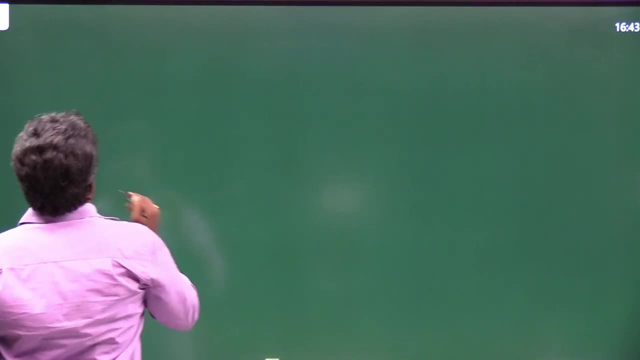 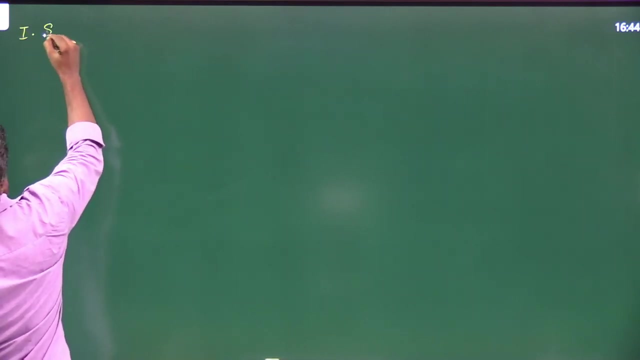 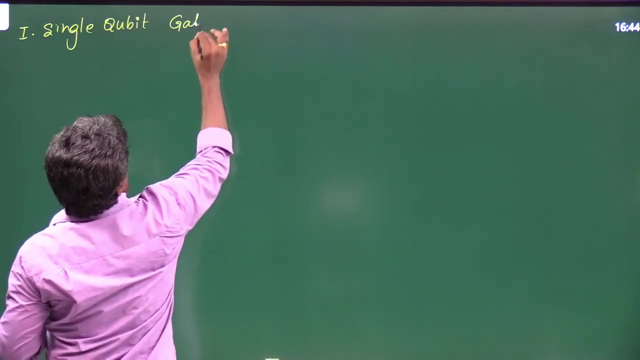 Now ready. So now we have completed this single qubit quantum gates. two qubit quantum gates and three qubit. Let me give you the conclusion. So please write all the things in one place. Now first one. So here I am taking single qubit, single qubit gates, quantum gates. Okay, So listen. 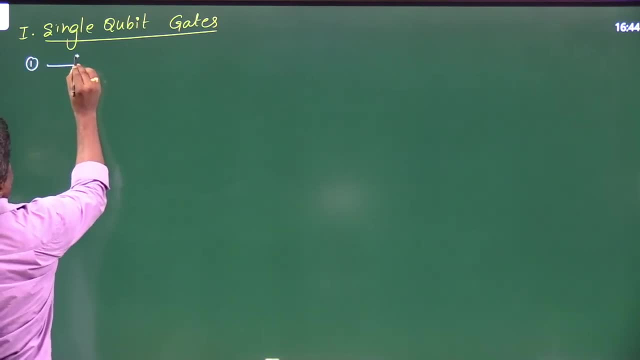 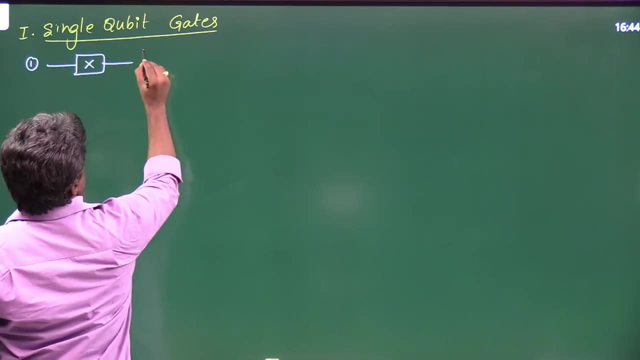 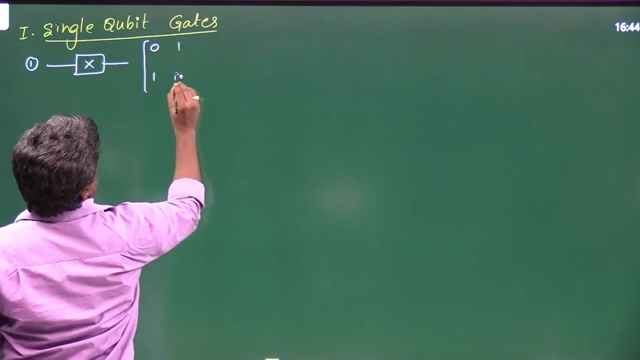 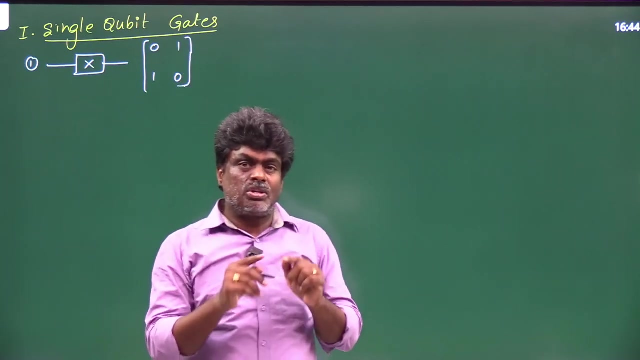 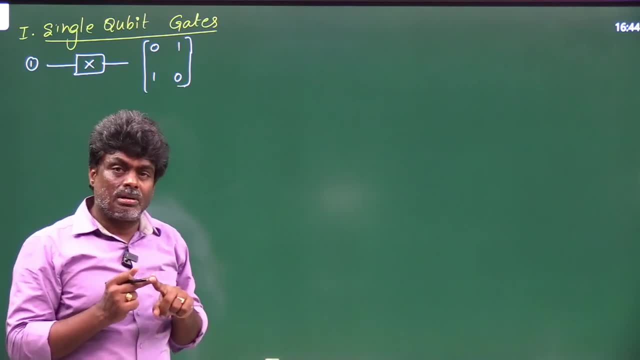 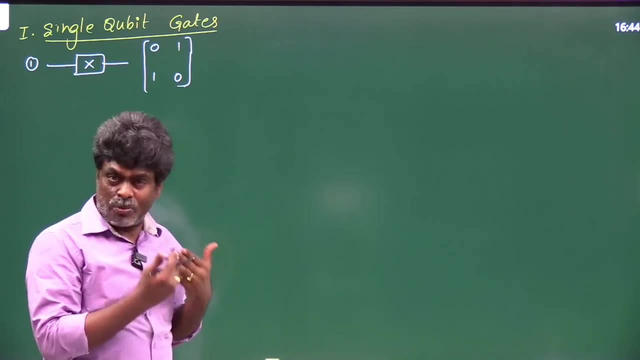 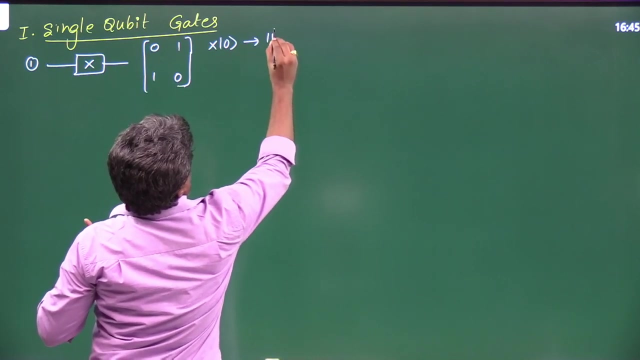 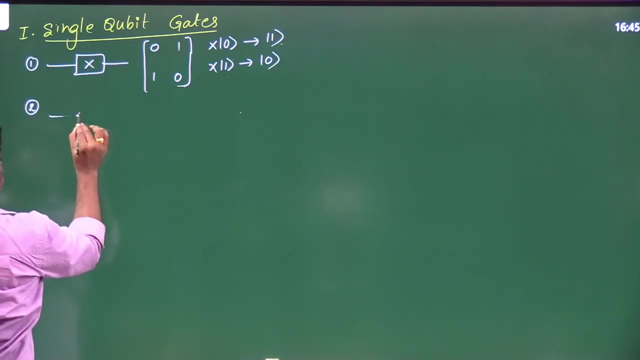 1: 0.. That means what this Pauli gate will do. It will interchange. It will interchange 0: 1 to 1, 0,, 1: 0 to 0: 1.. I hope you understand, That's it So, what it will do. This will interchange. That means 0 become 1 and 1 become 0.. Wait a minute, Next one. This is the Pauli y gate. First listen Few things, after that you can write. 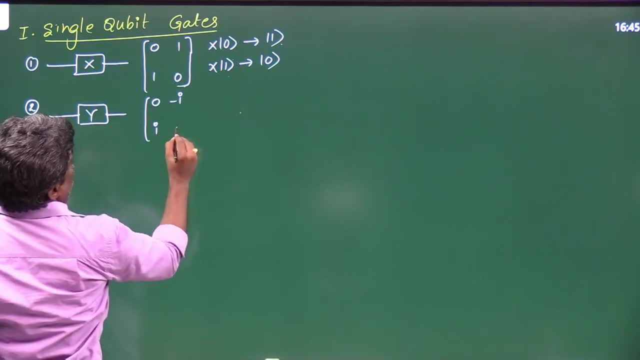 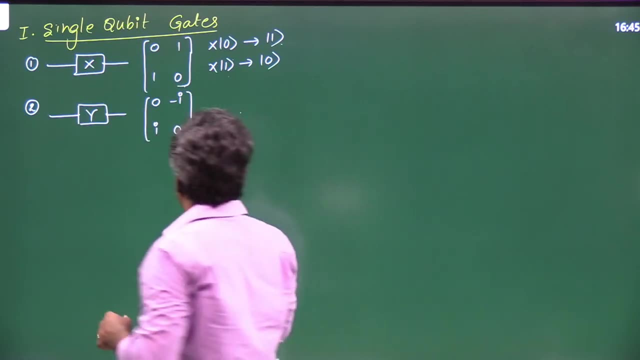 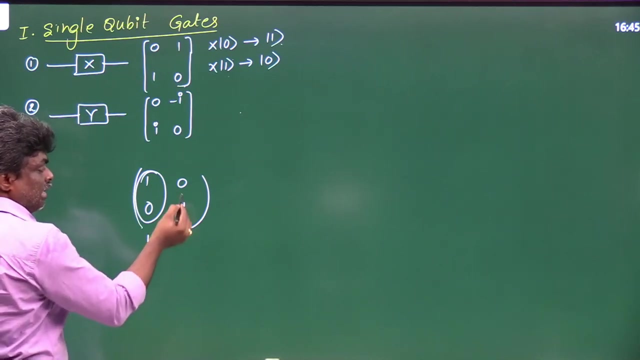 Now y gate is 0 minus i, i, 0.. Everybody Now just compare with the identity matrix: 1 0, 0, 1.. 1, 0, 0, 1.. Your 1, 0 is nothing but the 0. Okay Basis state And 0, 1 is nothing but the 1.. Now please compare, In the place of 1, 0, what you are having 0 i. That means y. 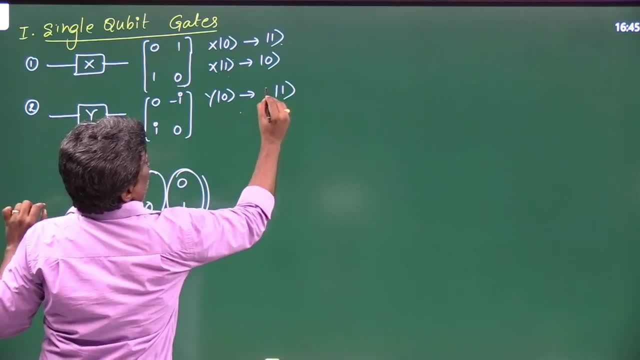 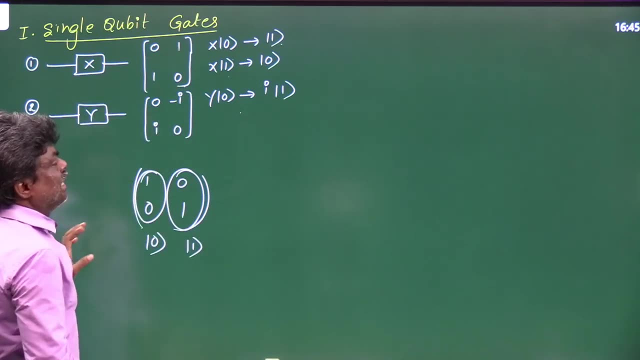 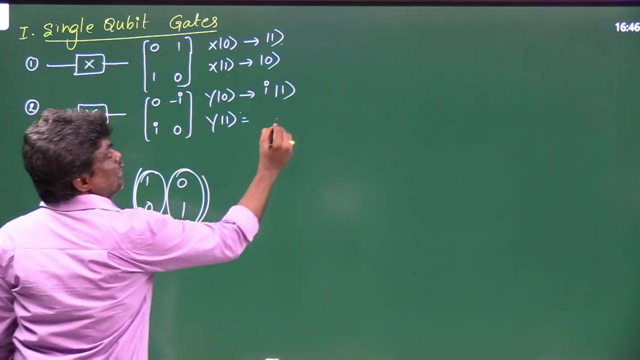 converts 0 to 1 with. i. No need to remember all these things, Very simple technique. Just compare with identity matrix. Next one: y operates on 1.. Now see the second column. So second column, actually what 0, 1.. 0, 1.. But 0, 1 become what Minus iota 0. That means it becomes 0 with minus iota. I hope you understand. Still not understand. 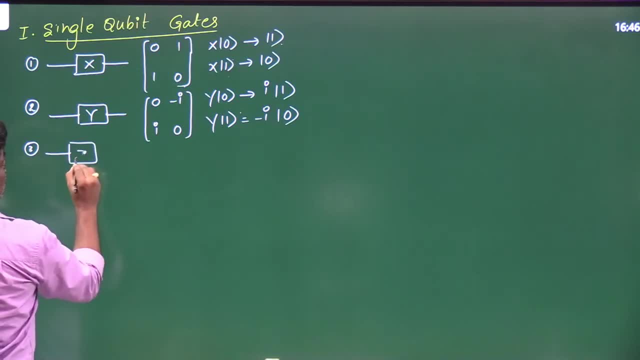 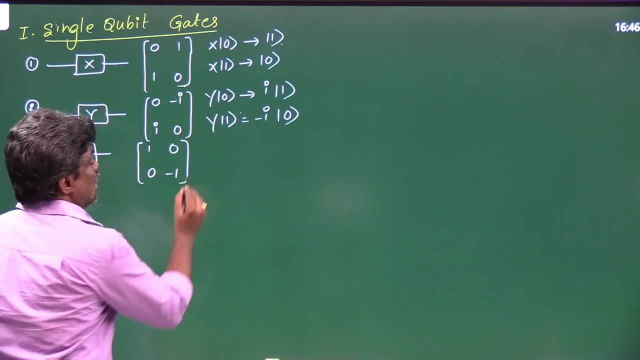 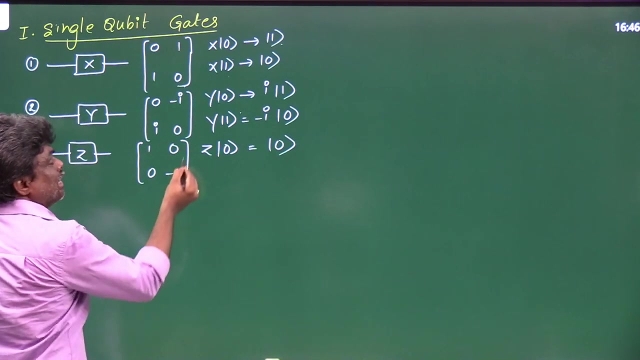 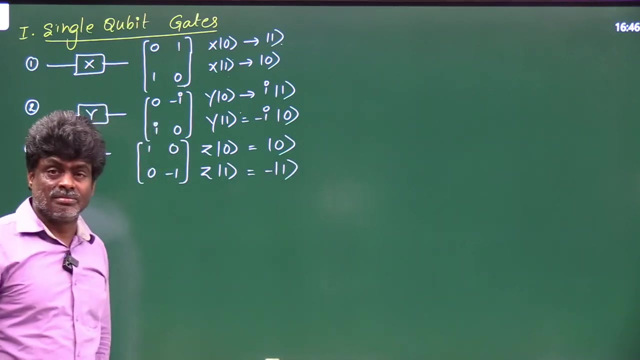 Third one. So this is the Pauli z gate. Could you please tell me 1, 0, 0 minus 1.. Now compare with the identity matrix. Luckily you have 1- 0. That's why no change. But in the place of 0- 1, you have 0 minus 1.. That's why it will convert minus 1.. Easy to remember. Next, fourth one: Head mod. 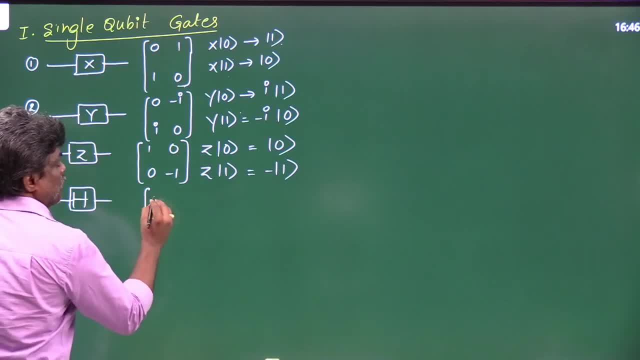 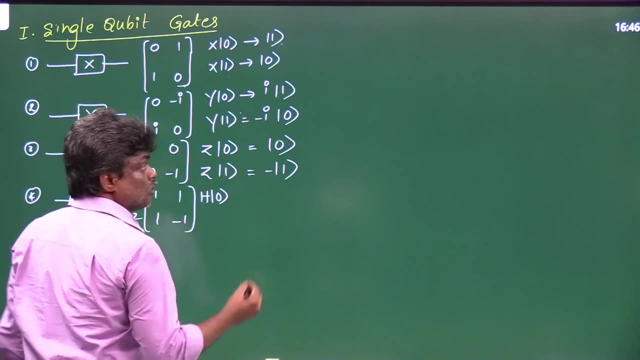 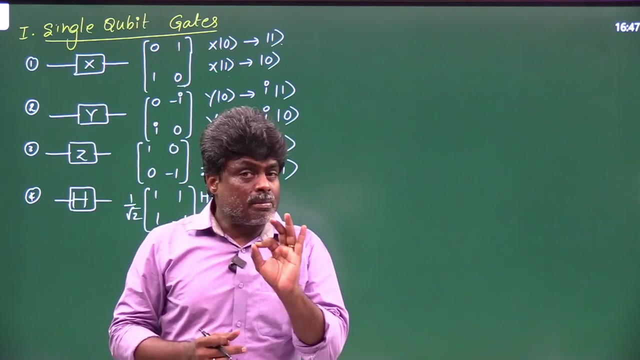 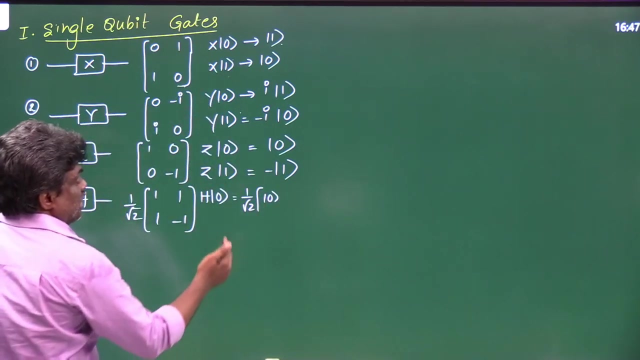 This is the representation of head mod gate. And what is operator 1? 1. 1 minus 1. 1 by root 2.. So head mod will give you the linear superposition, Not bell state, Not bell state. Bell state is also superposition state, But the head mod gate will give you simply superposition state, That is 1 by root, 2.. If you understand, you can start Plus 1.. How I am writing. 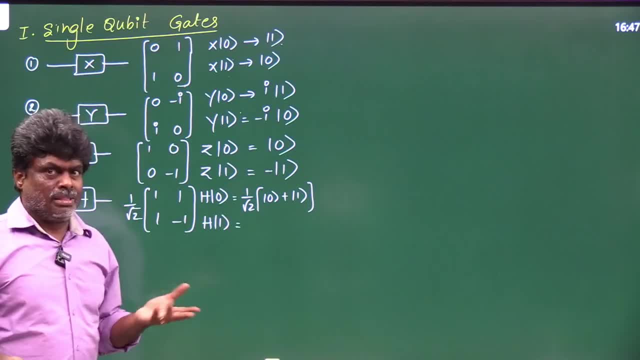 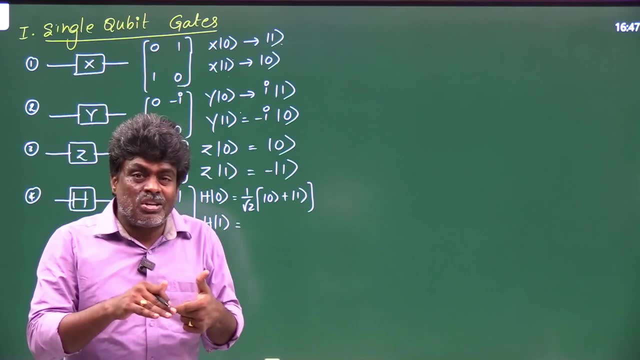 Sir, please tell You didn't say about this matrix, I think here, In the place of 1: 0, what you are having- 1, 1 you are having. That means it is converting 0 to 1: 1.. Once again, 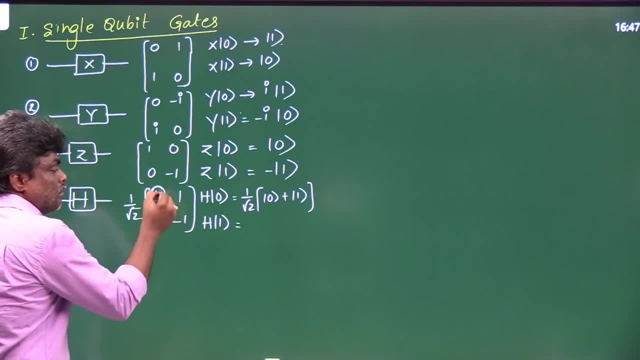 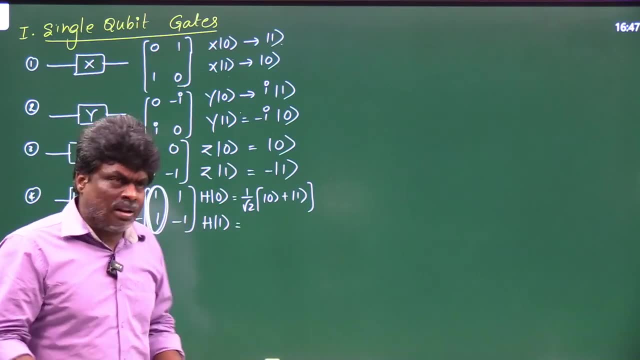 In the place of 1: 0.. This is my technique. In the place of 1: 0, you have 1: 1.. That means it is converting 1: 0 to 1: 1.. 1- 1.. In the place of 0: 1, it is having 1 minus 1.. 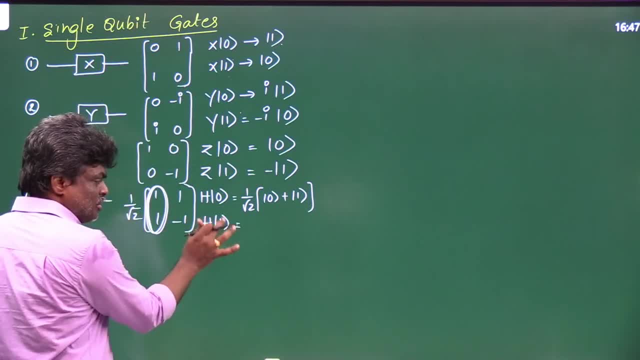 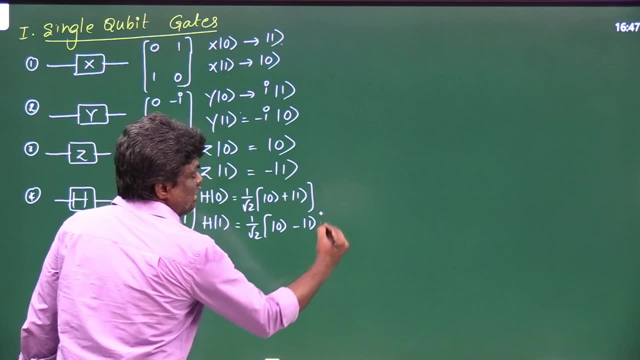 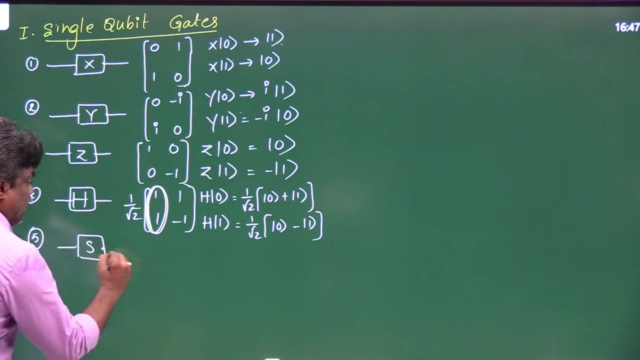 That means what It is converting: 0, 1.. 0, 1 state is nothing but 1.. It is converting 1 minus 1.. I hope you now you understand. Come on, And 5th one. This is the S gate. 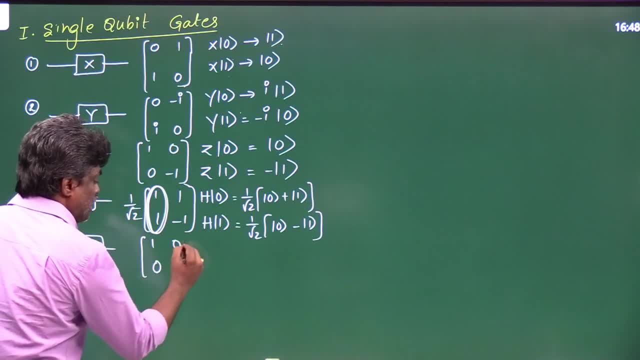 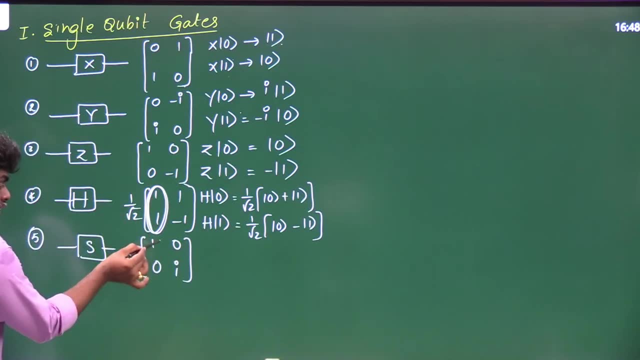 Which is 1, 0, 0 iota. So you please write. You please write, Don't multiply, Just apply the technique: 1: 0 as it is, Because 1, 0.. identity matrix: as it is no change, but 0i, please do it. and t gate. t is nothing but a square root. 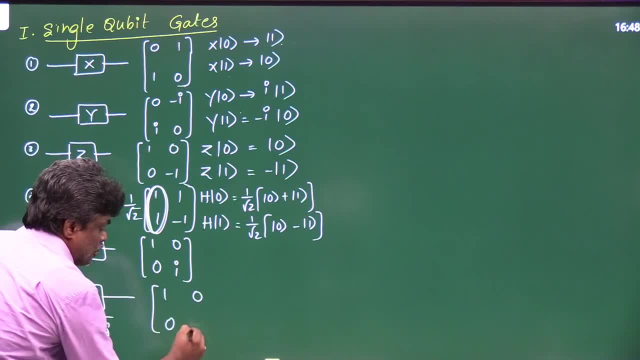 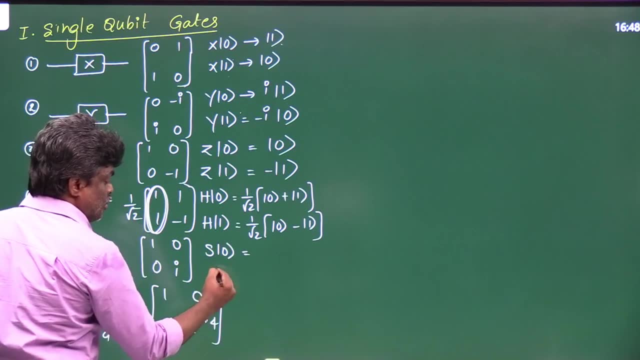 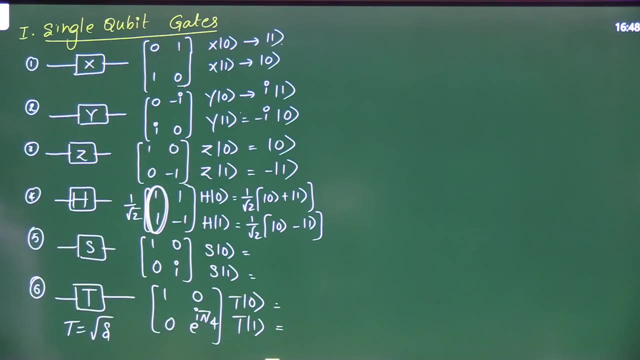 of s 1, 0, 0 e raised to i pi by 4, so s app operates on 0, s operates on 1, t operates on 0, t operates on 1. it's a very simple technique to identify what is the operation, just compare with identity. 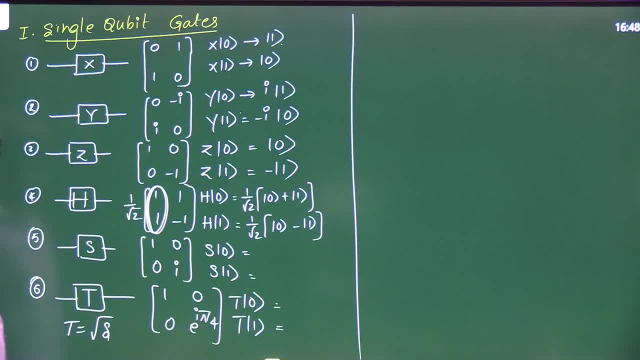 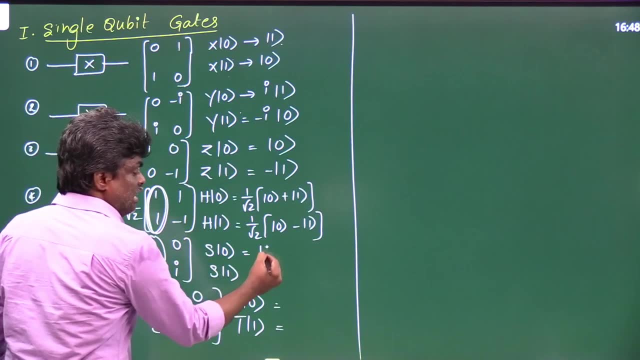 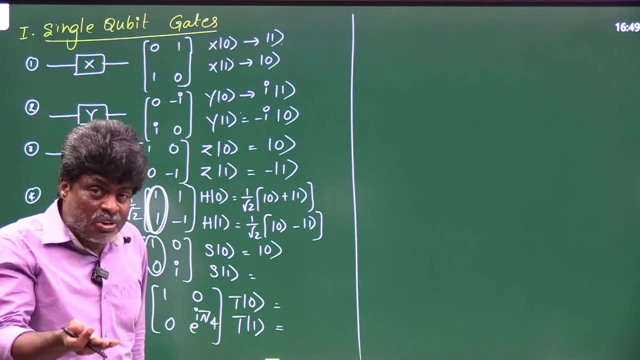 matrix. if you still not understanding, see in the identity matrix what you are having: 1, 0. here also 1, 0, no change. next 0, 1. but here you have 0 iota. that means it converts 0: 1 to 0 iota. that is i. 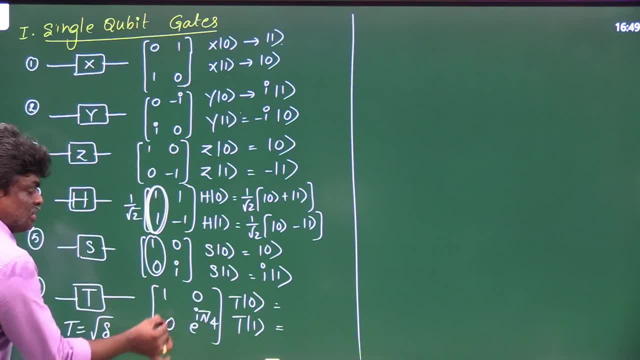 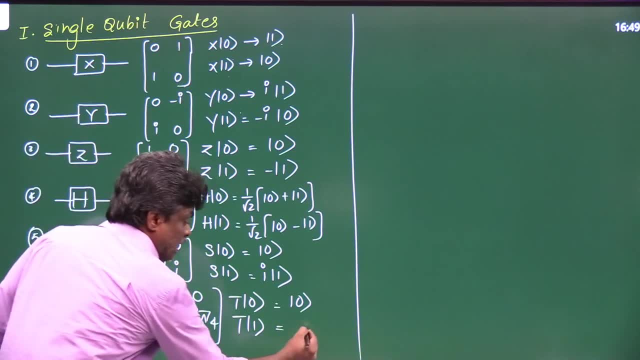 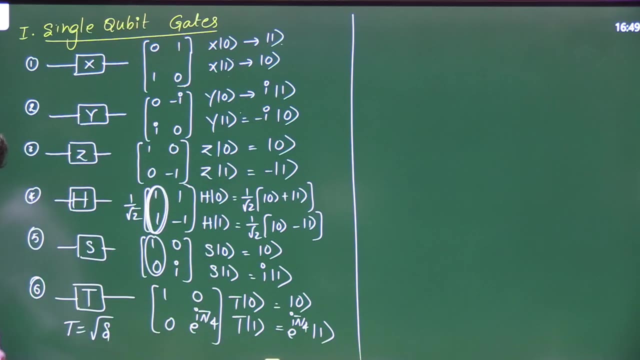 1. next here 1: 0. that's why as it is. but here 0, e raised to i power i pi by 4. that's why it converts 1 into e raised to i pi by 4. very simple: originally 0, 1 that is converted to 0, e raised to i pi by 4. 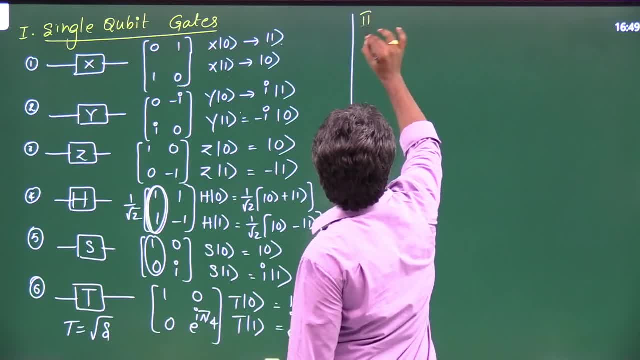 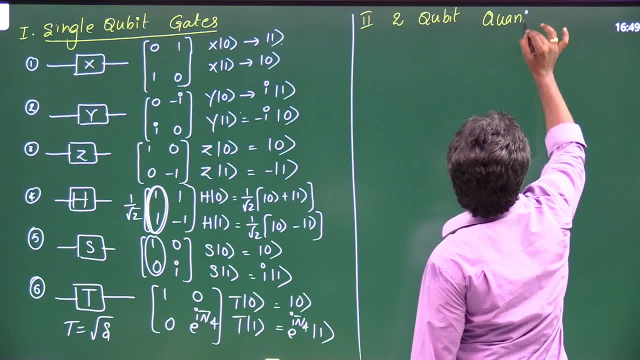 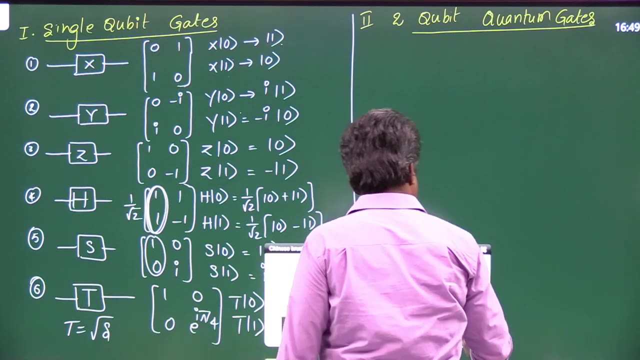 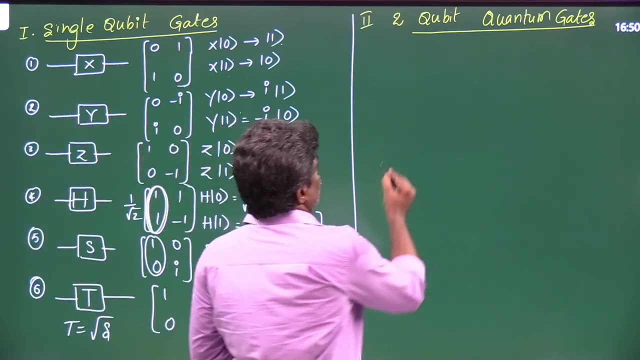 next, next, 2 qubit, second one: 2 qubit quantum gates. right, all the things at one place: 2 qubit, quantum gates. so this is the operation represented by cu- controlled unitary operation. so this is the operation represented by cu- controlled unitary operation. 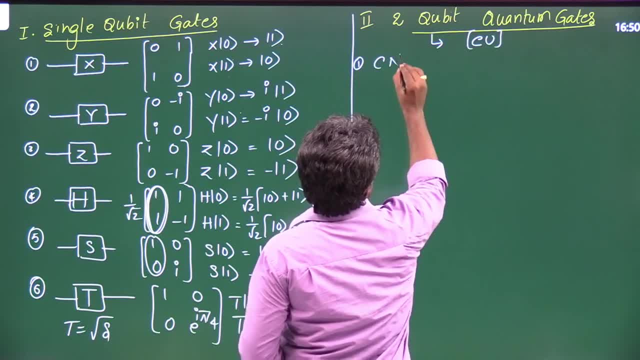 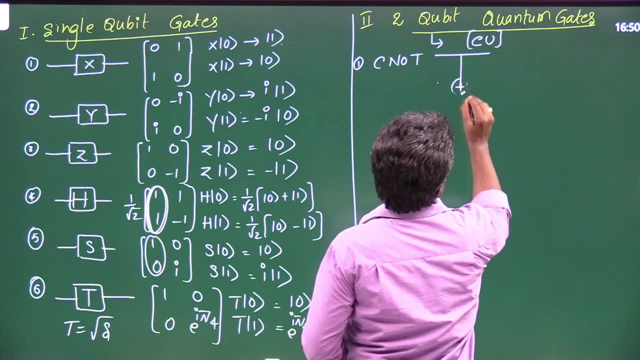 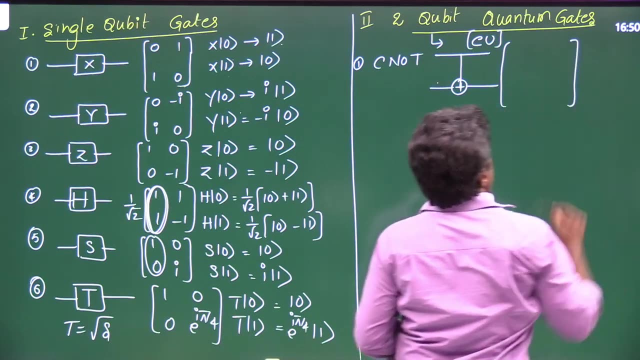 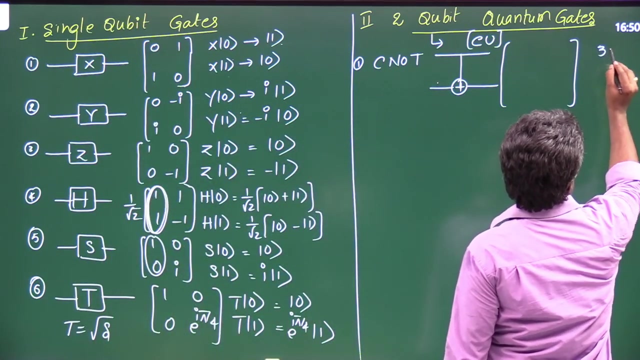 so this is the operation represented by cu, controlled unitary operation. first one, Christina, how to represent you know 222. present the gate and give them at race and tube operation as a- I hope you know that- and give operation anybody now it converges it cop合ه. 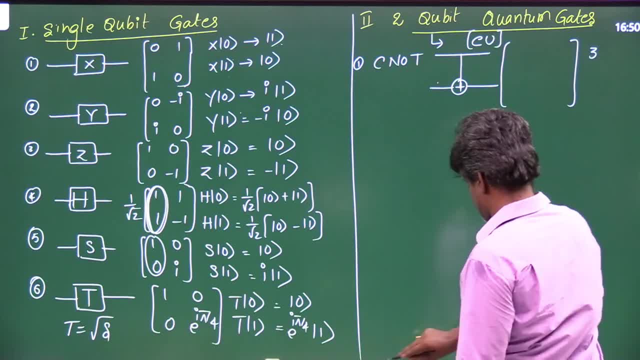 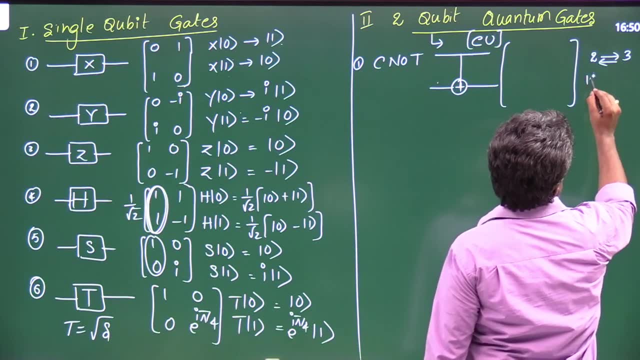 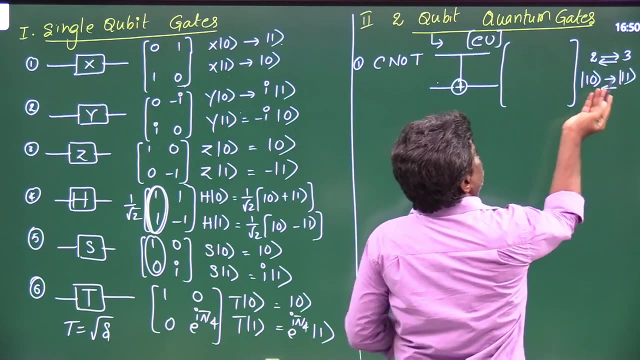 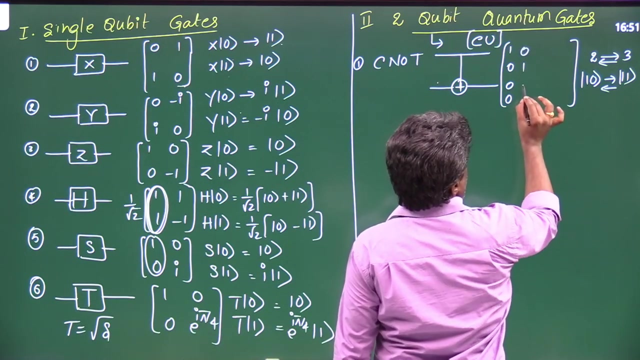 223, 223, 3. sorry, it converts 2, 2, 3, 3, 2, 3, 2, 2. that's why 1: 0 converts to 1, 1 and vice versa. that means second and third column are interchanged. first: 0 column- no change. next column: no change: 1. this is. 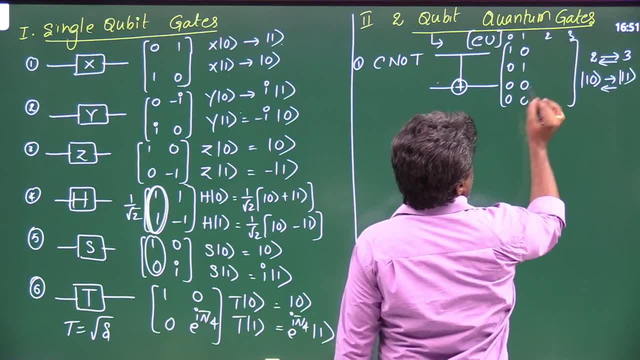 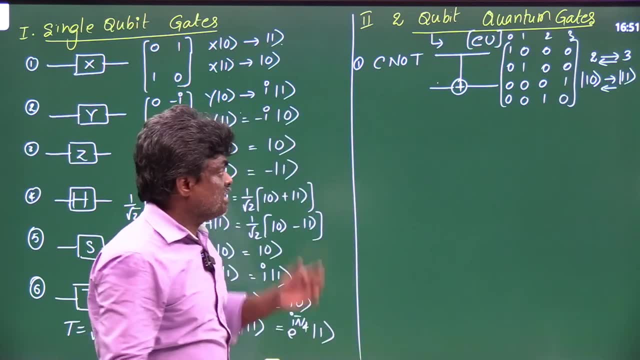 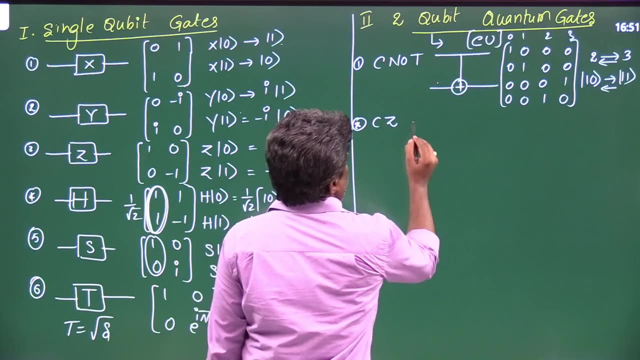 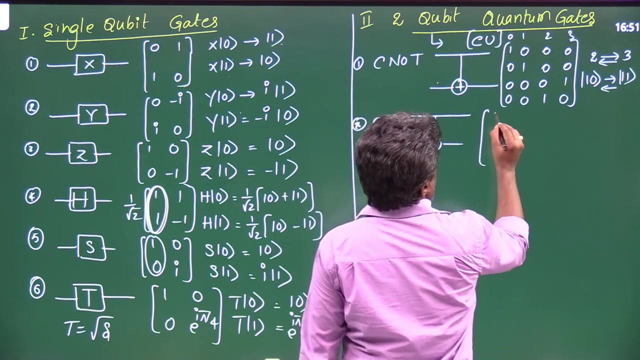 0, 1, 2, 3, no change, but here interchanged, no confusion at all. please write yourself. and the second one CZ. so CZ, I hope you can write directly: this is 1 0 0, 1, because I 0 0 0, 0, if you. 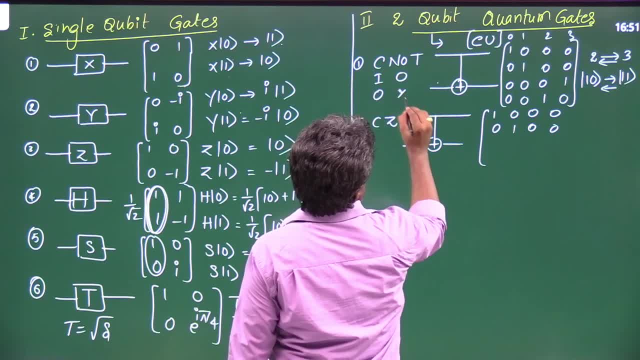 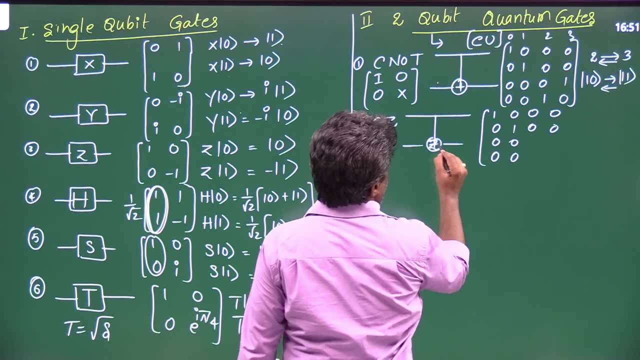 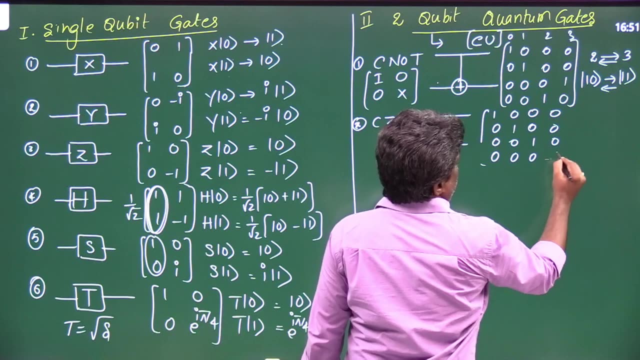 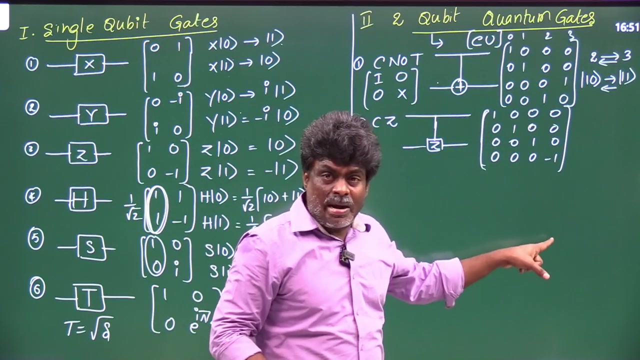 have confusion. you can write like this also: this is the matrix, so 0 0 0, 0 here. sorry, here we have Z. I'm sorry, this is the Z, so Z is 1 0 0 minus 1. now no need to remember anything, just follow my technique. compare with identity matrix. 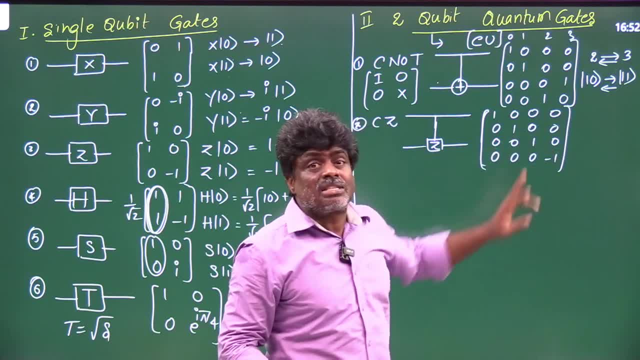 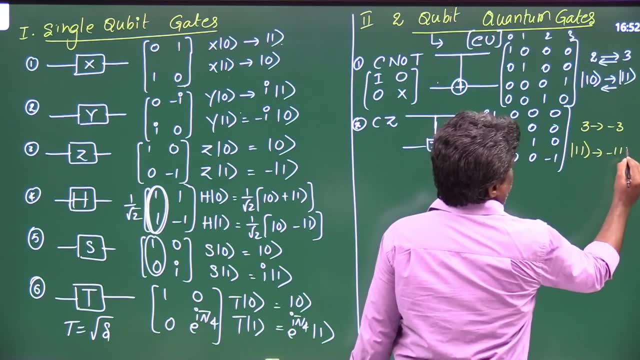 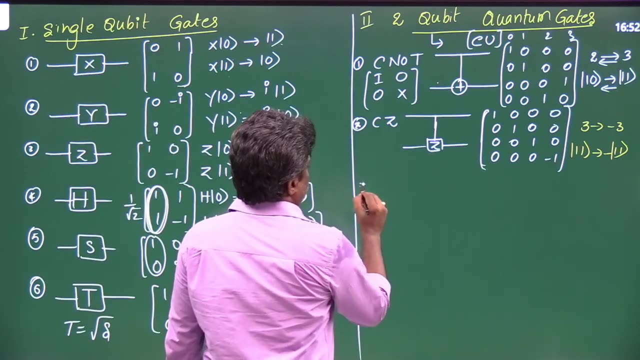 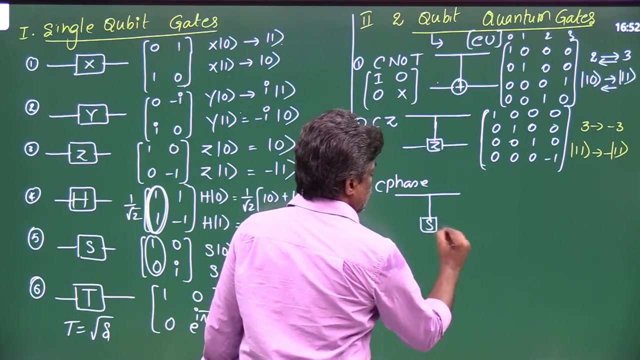 no change, no change, no change. the last one, last one is a: 3: 3 become minus 3, that is 1: 1 become minus 1, 1. I hope now you understand. next third one: C phase. so this is yes and this is I hope you know I, so I.